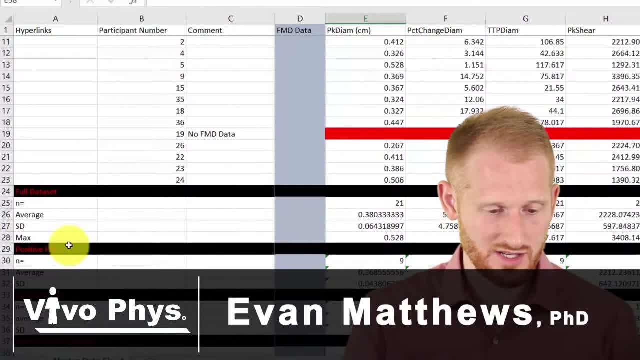 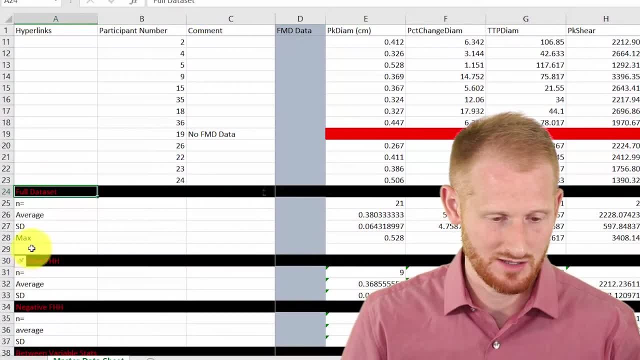 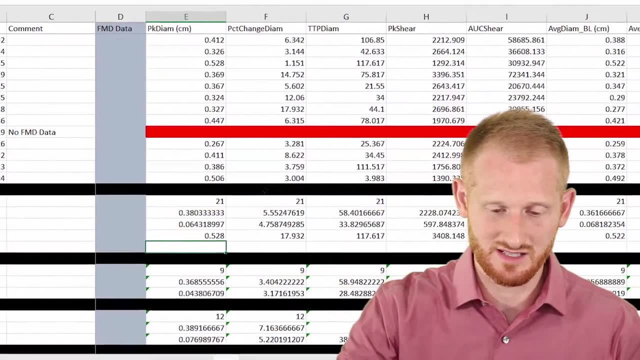 So let's add minimum data points to our data sheet here. So let's add in another row underneath of our full data set, statistics section. So I'm going to type min here for minimum and let's go to where we want the minimum statistic to be calculated. Hit the equal sign m-i-n for minimum and double. 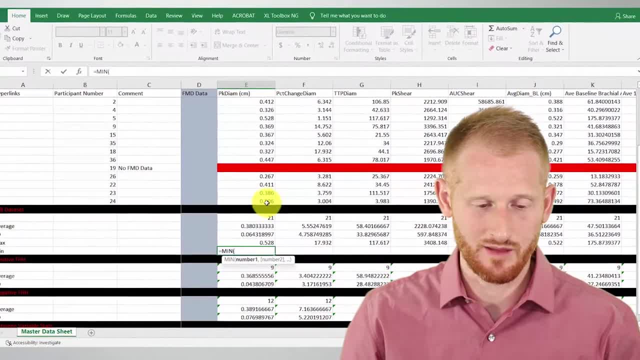 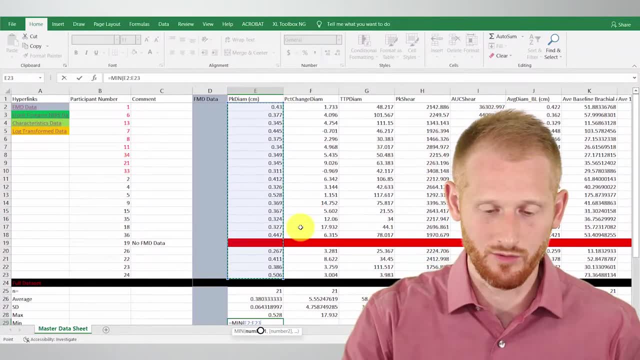 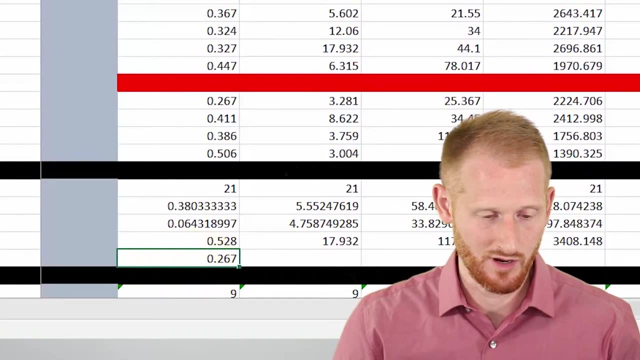 click this first one that pops up. Now, since I'm doing it for the full data set, I'm going to highlight all of the data in that column for the full data set, regardless of what group they're in, So whatever group the participants are in, and so our minimum value is 0.267.. We had already 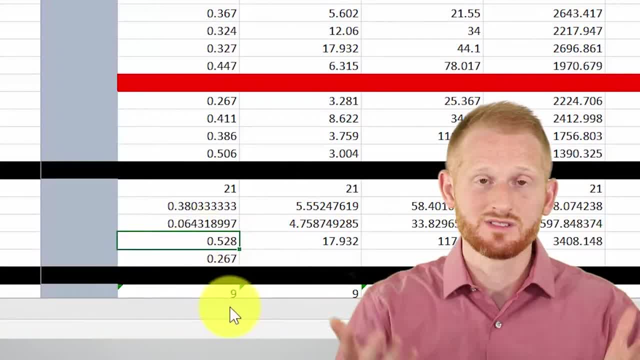 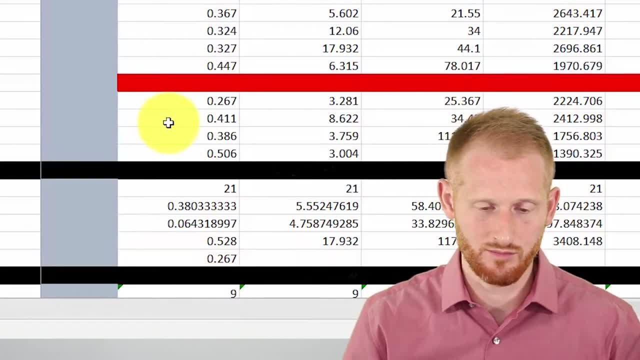 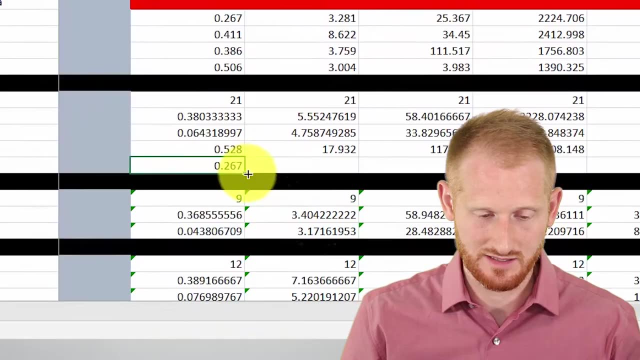 calculated, our maximum value is 0.528.. So our range then is 0.627 to 0.528 for the peak diameter. This is brachial artery diameters for our data set, and so let's go ahead and click that at that minimum that we just calculated. Let's drag that across by going to the little box in. 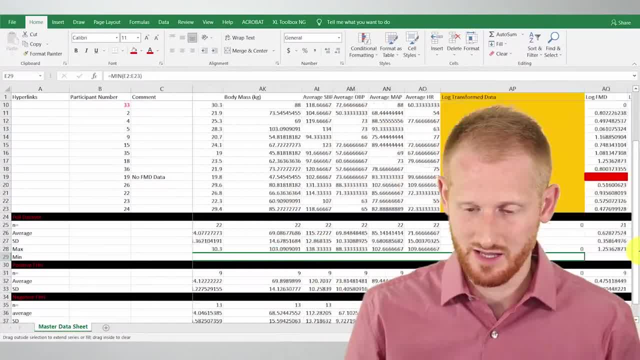 the bottom right corner, getting that cursor as a plus and dragging it across all of our columns of data. so we have our minimum calculations for every data set.